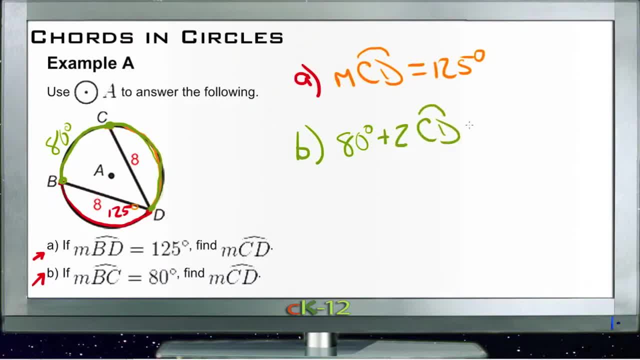 so two times CD is equal to 360 degrees, because that's the whole circle. then we can just subtract the 80 degrees from both sides: 360 minus 80 is 280, and then we know that two times CD is equal to 280 degrees. so we divide both sides by: 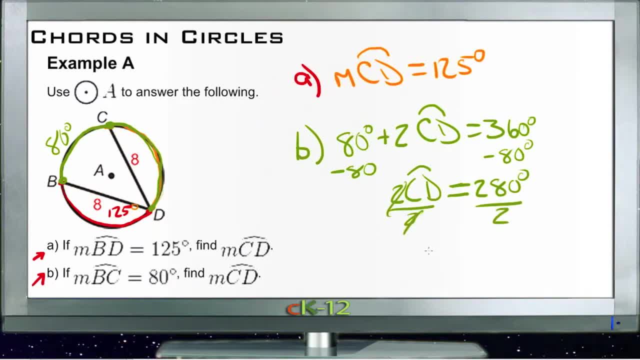 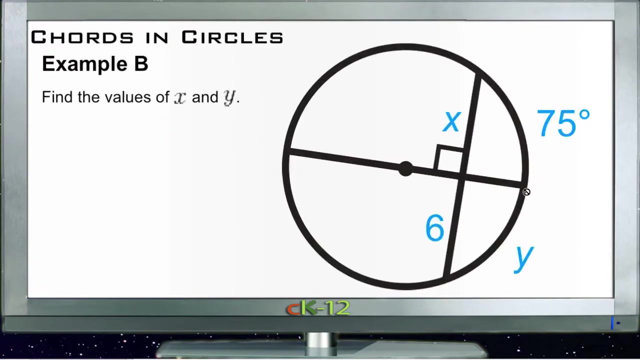 two and we get: CD is equal to half of 280 or 140. so you can see in the second question here, in part B, CD is 140 degrees, whereas in the first part it was 125 degrees. so don't let that confuse you. alright, example B. example B says: find the values of X and Y. so X is this. 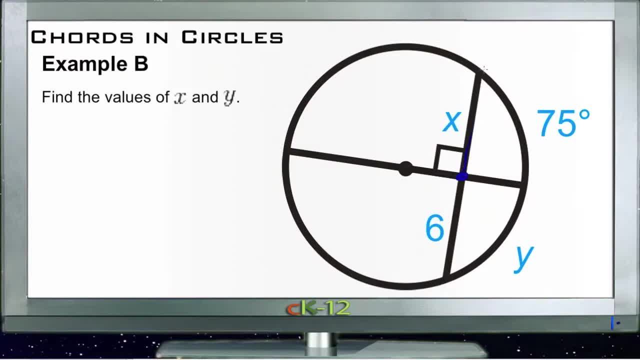 portion of this chord, which that's not a very good color for that. let's try that again. X is the upper portion of this chord right here, the chord that goes all the way across, and since this line right here is a diameter, we know that the diameter meeting at 90 degrees- so it's perpendicular- bisects this chord, so that 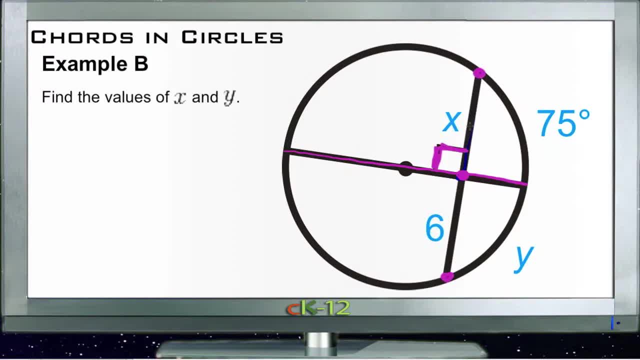 tells us that X and six are equal halves of the same chord, so that X and six must be the same thing. so that tells us that X equals six, then Y is similar. we have that same diameter meeting at a 90-degree angle or perpendicular to the 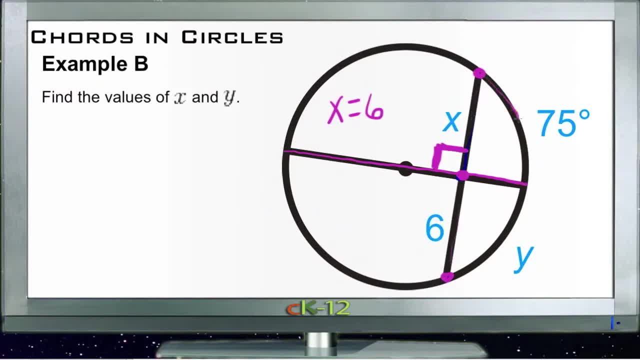 chord and that cord describes this arc right here. so that diameter then bisects that chord, which tells us that 75 and Y are equal halves of this arc right here. so now we know that Y is equal to 75 degrees. easy enough, okay. and then example: 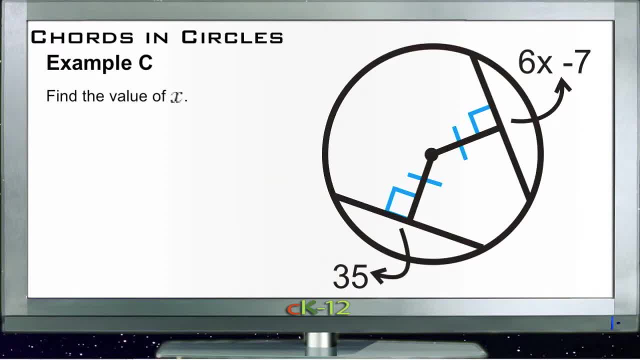 see example. see says: find the value of X. well, this one's actually easier than it looks, because we have this information right here that tells us that this chord right here, or this, what would be a radius if it goes all the way out, this radius right here?